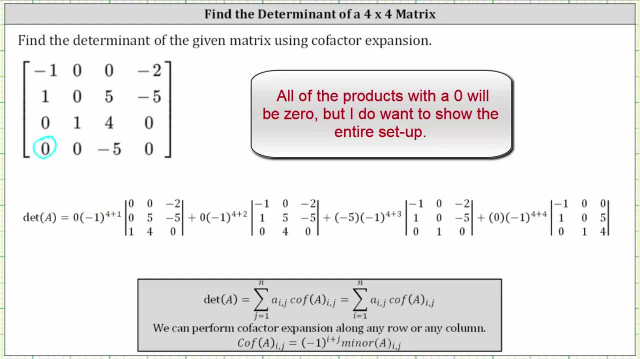 Next, we eliminate row four and column one from the matrix, and multiply by the determinant of the remaining matrix. Notice how we have a three by three matrix where the first row is zero, zero, negative two, the second row is zero, five, negative five, the third row is one, four, zero. So we have the three by three determinant of this matrix shown here. So here we have a sub four comma one times the corresponding cofactor. 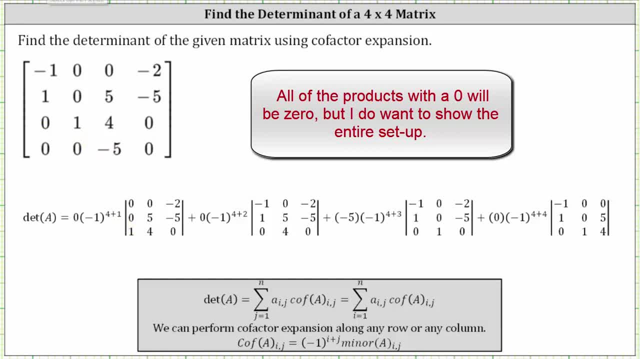 And now you move along to the next element in row four. So we have plus, next element is zero, and this element is in row four, column two. And therefore we multiply by negative one, raise the power of four plus two. And then we multiply by the determinant of the matrix formed by eliminating row four and column two. 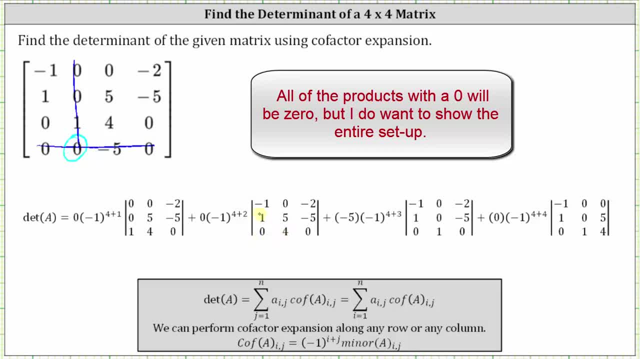 Notice how that gives us the three by three determinant shown here, where the first row is negative one, zero, negative two. 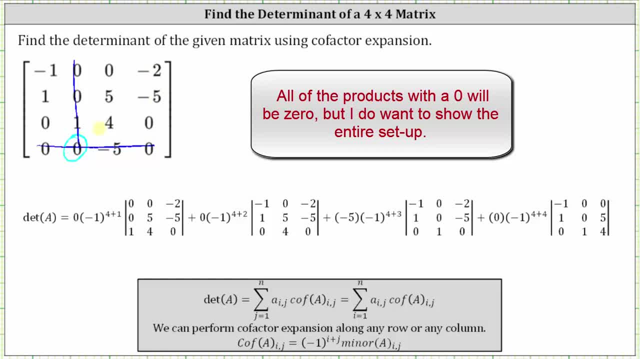 The second row is one, five, negative five. And the third row is zero, four, zero. 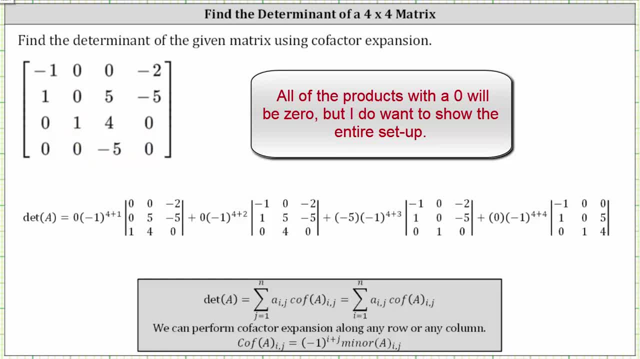 And we move on to the next element, in row four, which is the element of negative five in row four, column three. So we have plus negative five times negative one, raise the power of four plus three. Again, four plus three is the exponent because the negative five is in row four, column three. 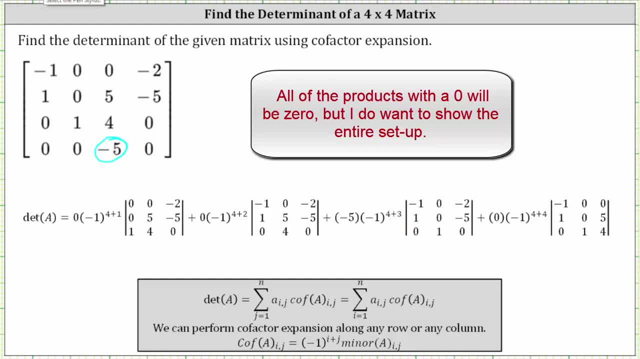 And then we multiply by the determinant of the matrix formed by eliminating row four and column three, which gives us the three by three determinant shown here, where the first row is negative one, zero, negative two, the second row is one, zero, negative five. And the third row is zero, one, zero. 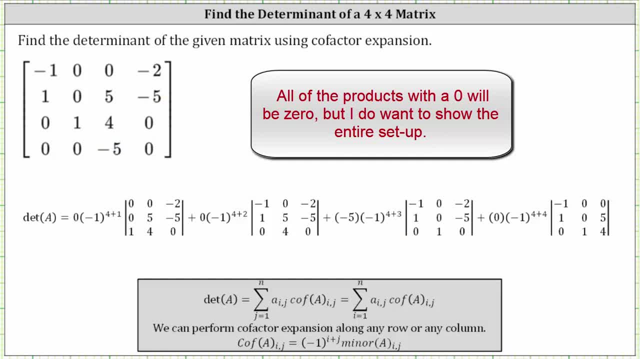 Now we move on to the last element in row four, which is the element in row four, column four, which again is another zero. 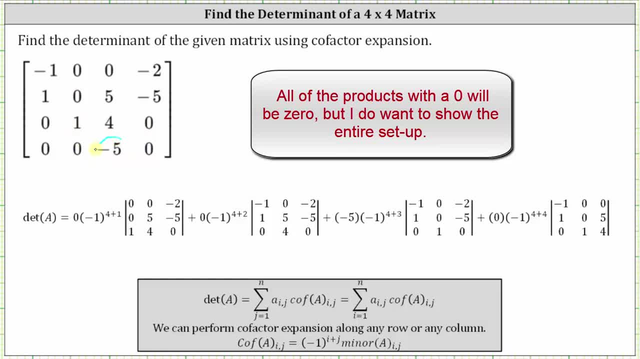 in row four, which is the element of negative five in row four, column three. So we have plus negative five times negative one. raise the power of four plus three. Again, four plus three is the exponent because the negative five is in row four, column three. 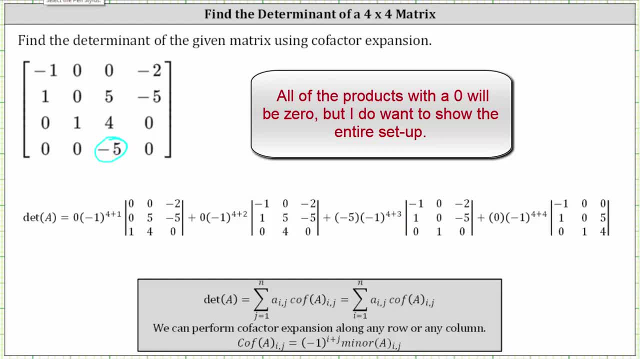 And then we multiply by the determinant of the matrix formed by eliminating row four and column three, which gives us the three by three determinant shown here, where the first row is negative one- zero negative two- the second row is one- zero, negative five. 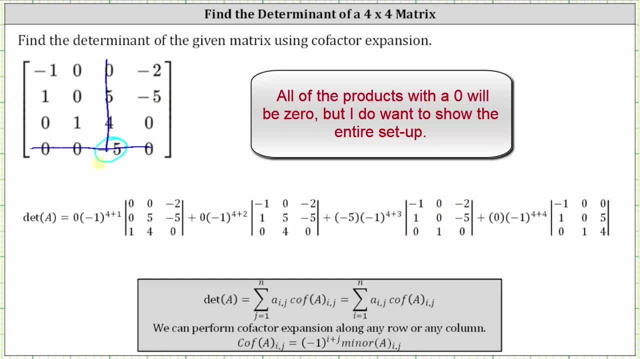 and the third row is zero, one zero. Now we move on to the last element in row four, which is the element in row four, column four, which again is another zero. So we have plus zero times negative one. raise the power of four plus four. 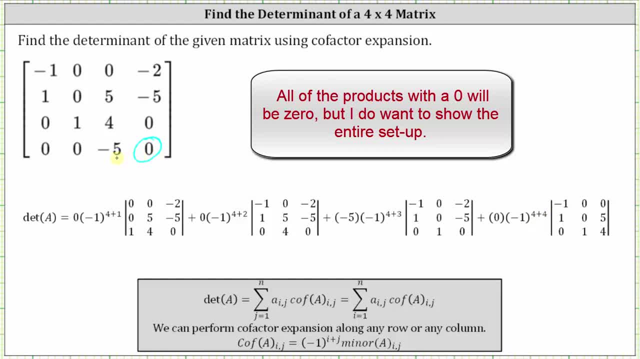 Again, the exponent is four plus four, because the element is in row four, column four. Then we multiply by the determinant of the matrix formed by eliminating row four, column four, which leaves us with a three by three determinant, shown here, where the first row is negative: one, zero, zero. 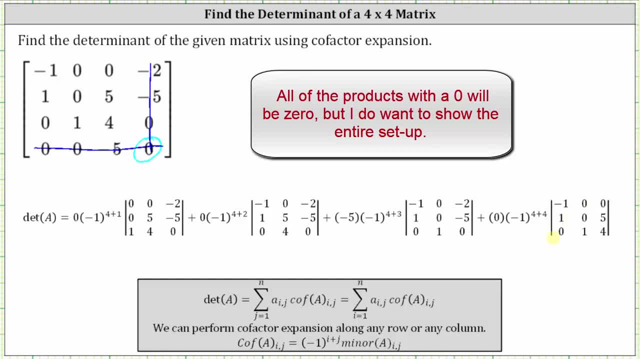 the second row is one zero five. and the third row is zero one four. Now, the reason we selected row four is because three of these products contain a zero, reducing the amount of work that we have to do. This first product is zero. the second product is zero. 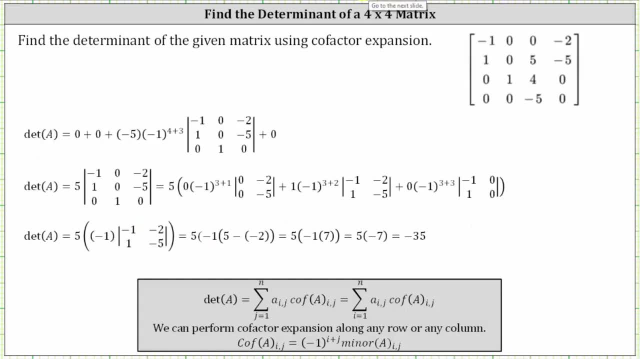 and the fourth product is zero, which gives us zero plus zero, plus negative five times negative one. raise the power of four plus three times the three by three, determinant plus zero. So of course we can drop the zeros And since negative five times negative one. 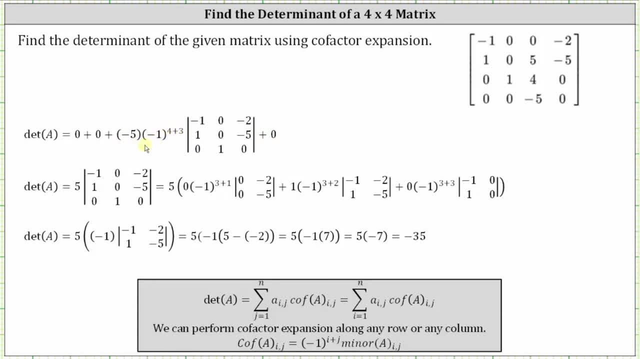 raise the power of seven is equal to positive five. we are left with positive five times the three by three determinant. So now we need to evaluate this three by three determinant, And again we'll use the method of cofactor expansion, Because row three has two zeros. 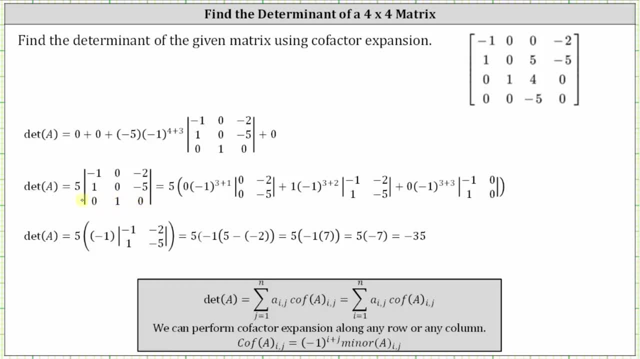 we will perform cofactor expansion along row three. Now we need to be careful here. It's going to be five times the value of this determinant. So we have five and then an open parenthesis, And then the element in row three, column one, is a zero. 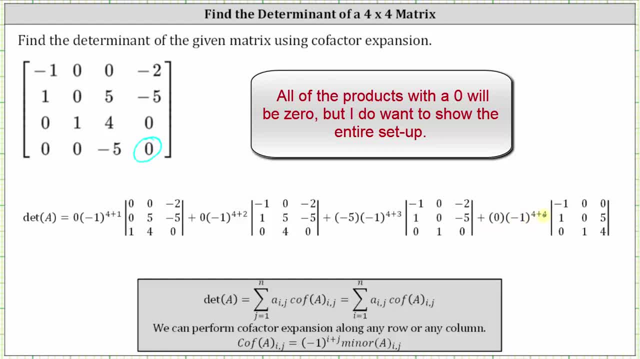 So we have plus zero times negative one, raise the power of four plus four. Again, the exponent is four plus four because the element is in row four, column four. Then we multiply by the determinant of the matrix formed by eliminating, row four, column four, which leaves us with a three by three determinant shown here, where the first row is negative one, zero, zero, the second row is one, zero, five, and the third row is zero, one, four. 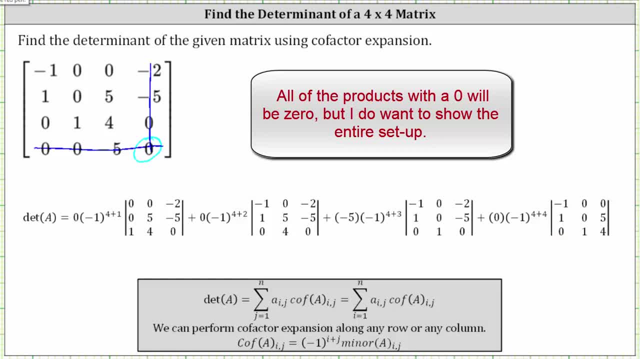 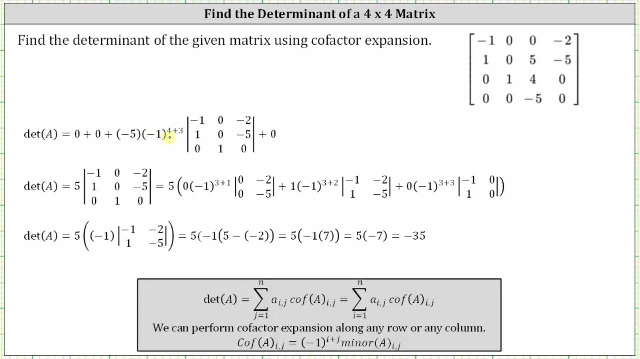 Now the reason we selected row four is because three of these products contain a zero, reducing the amount of work that we have to do. This first product is zero, the second product is zero, and the fourth product is zero, which gives us zero plus zero plus negative five times negative one raised to the power of four plus three times the three by three determinant plus zero. 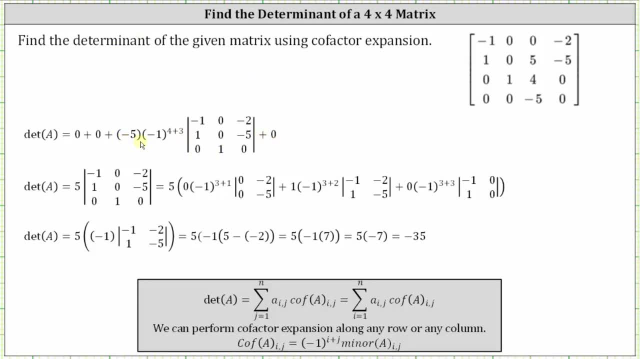 So of course, we can drop the zeros, and since negative five times negative one raised to the power of seven is equal to positive five, we are left with positive five times the three by three determinant. So now we need to evaluate this three by three determinant, and again, we'll use the method of cofactor expansion. Because row three has two zeros, we will perform cofactor expansion and we will perform cofactor expansion. 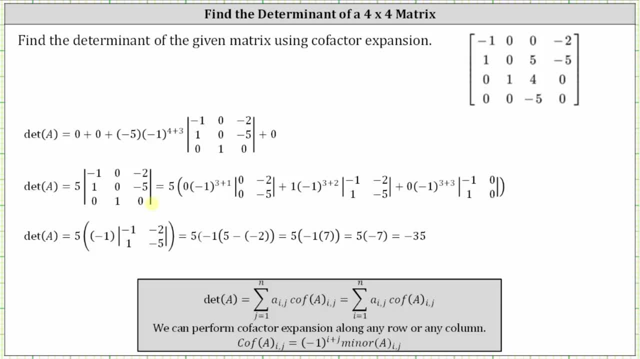 along row three. Now we need to be careful here, it's going to be five times the value of this determinant, so we have five and then an open parenthesis, and then the element in row three column one is a zero, so that's why we have a zero here, times negative one raised to the power of three plus one, because the zero was in row three column one. Next we eliminate row three column one, which gives us a two by two determinant shown here, where the first row is zero negative two, and the second row is zero negative five. 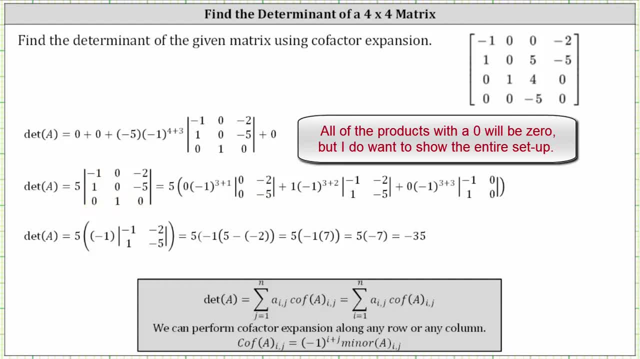 Now we move along to the second element in row three, which is a one, 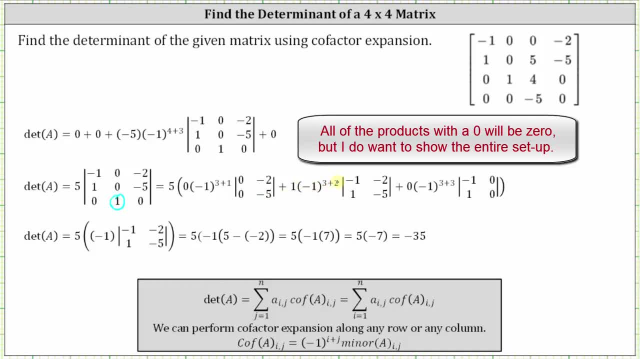 which gives us plus one times negative one raised to the power of three plus two. The exponent is three plus two because the element of one is in row three column two. 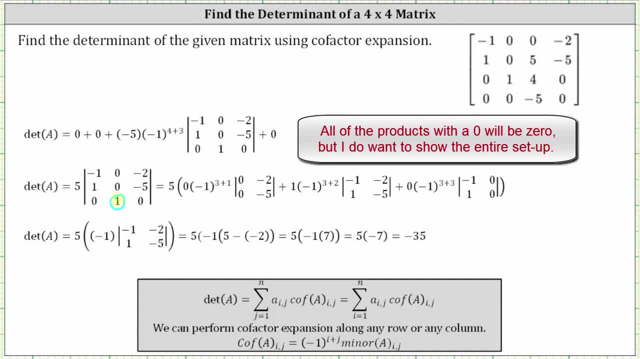 Next we eliminate the row and column of this element, or row three and column two, which gives us a two by two determinant, where row one is negative one negative two, the second row is one negative five. 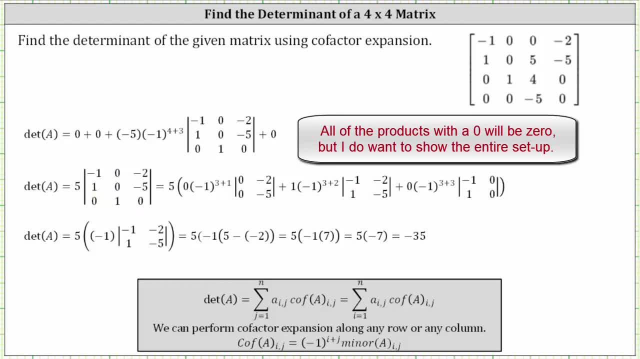 We move along to the last element in row three, which is the zero in row three column three, so we have plus zero times negative one raised to the power of three plus three, and we eliminate the row and column of this element, or row three and column three, which gives us the remaining two by two determinant, where the first row is negative one zero, and the second row is one zero. 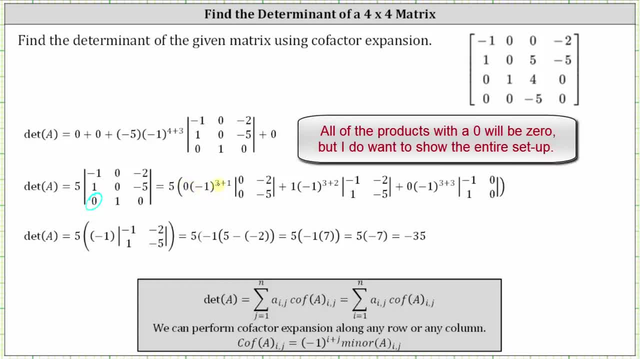 So that's why we have a zero here. Times negative one raise the power of three plus one, because the zero was in row three, column one. Next we eliminate row three, column one, which gives us a two by two determinant, shown here, Where the first row is zero, negative two. 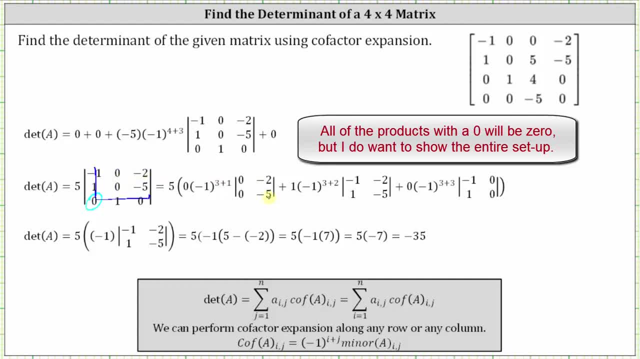 and the second row is zero negative five. Now we move along to the second element in row three, which is a one which gives us plus one times negative one. raise the power of three plus two. The exponent is three plus two because the element of one is in row three, column two. 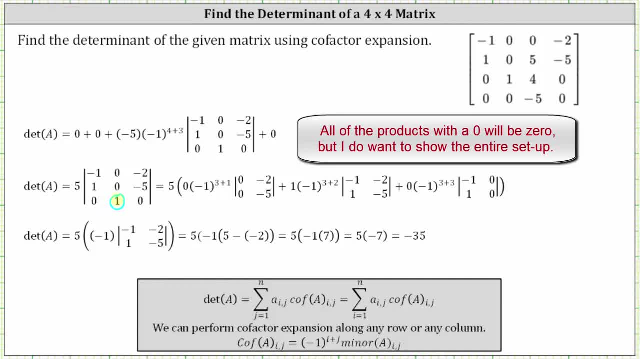 Next, we eliminate the row and column of this element, or row three and column two, which gives us a two by two Determinant. where row one is negative, one negative two, The second row is one negative five. We move along to the last element in row three. 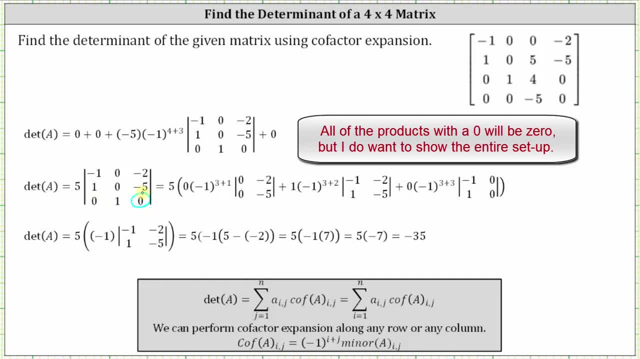 which is the zero in row three, column three. So we have plus zero times negative one raise the power of three plus three And we eliminate the row and column of this element, or row three and column three, which gives us the remaining two by two determinant. 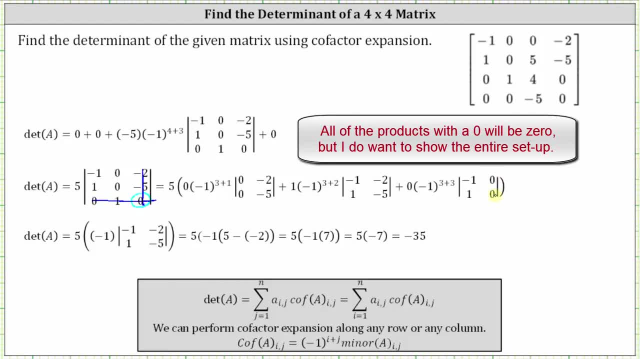 where the first row is negative, one zero and the second row is zero. so it's negative, one zero and the second row is one zero. So two of these three products will be zero. Notice how the first product has a factor of zero. 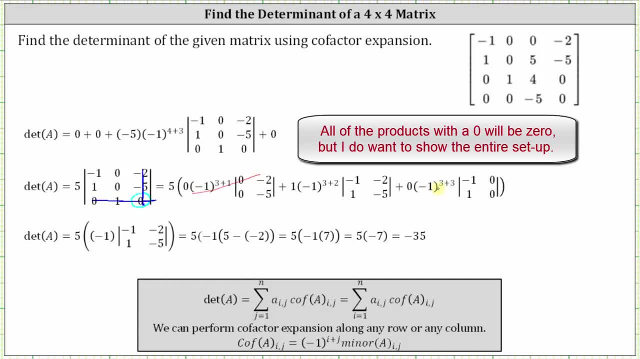 so this will be zero. and the third product has a factor of zero, so this will be zero. This leaves us with five, and then times negative one to the fifth power is negative one, so one times negative one is negative one. and then we have the two by two determinant. 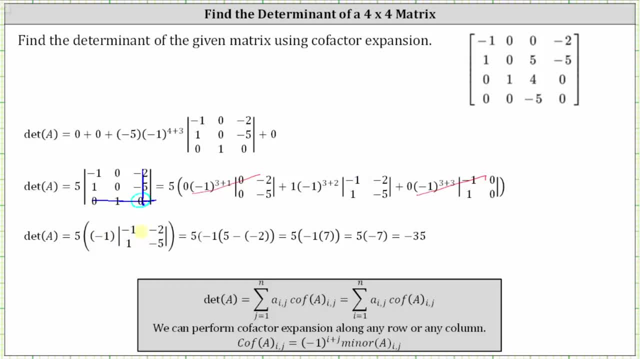 To evaluate the two by two determinant, we have the product of the main diagonal minus the product of the minor diagonal, which gives us five minus negative two. inside parentheses, Of course, five minus negative two is equivalent to five plus two or seven. 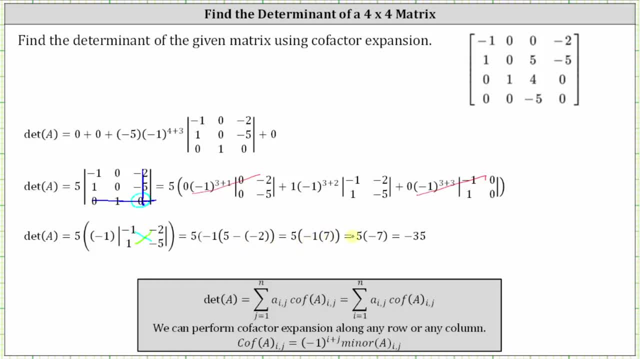 which gives us five times negative, one times seven, or five times negative seven, which is negative 35. So the value of the four by four determinant is negative 35. I hope you found this helpful.